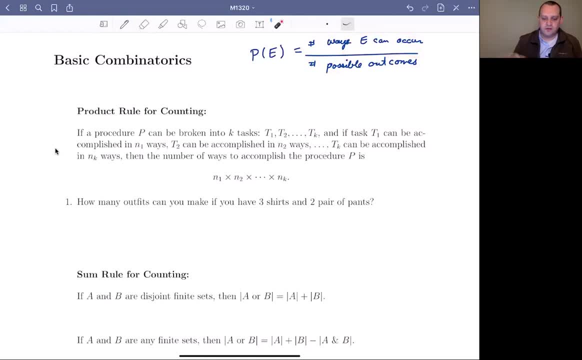 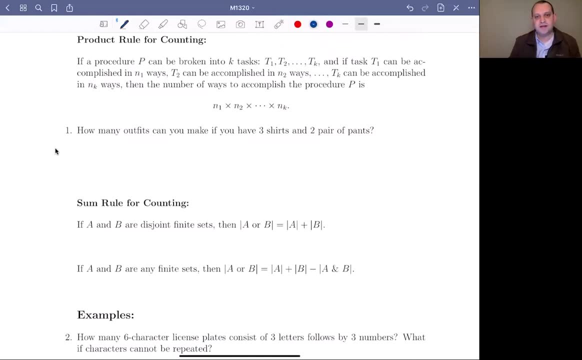 So there's two basic rules to start. The first is what's called the product rule for counting, not to be confused with the product rule from calculus. but the product rule for counting says that if you have some total operations that you can do in the first piece, you can do the third piece, and so on. 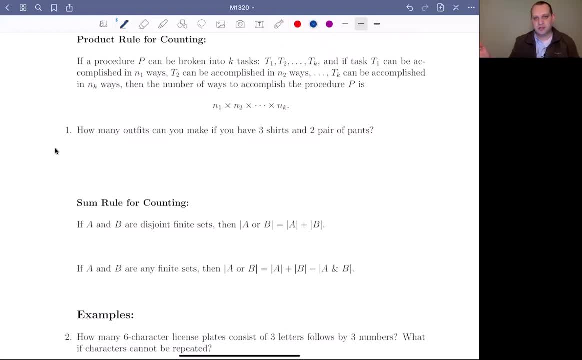 And the total number of ways that you can do this procedure is N1 times N2 times N3.. So it's the number of ways you can do the first piece times the number of ways you can do the second piece times the number of ways you can do the third piece, and so on. That's the product rule. 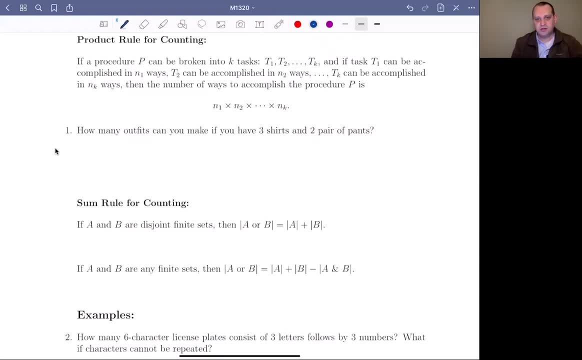 So the way I like to think about this is: let's say, you just have three shirts and two pair of pants and you want to make an outfit from the first piece to the second piece. So you can do the three pieces or you can make the i-pl wiped out of the linen. 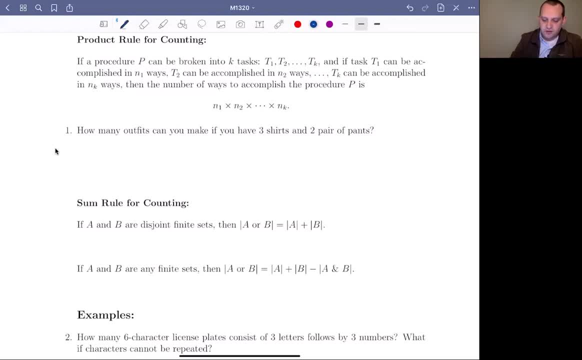 And then you want to know how many outfits can you make? Well, you have three choices for shirts, and then, for each choice of shirt, you have two pair pants. you have two options there And then each path, so each path here. if I go that way, that's one outfit. 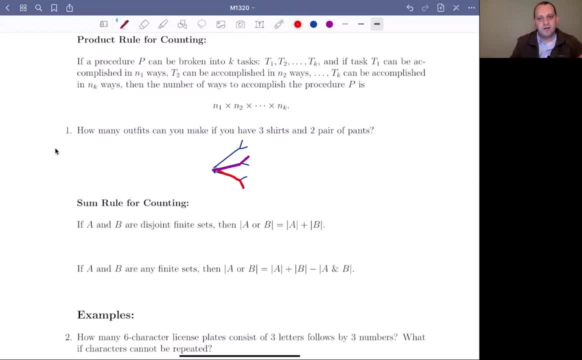 Here's another outfit, and so on. So how many total outfits are there? There's six, And six is three times two, So that's one outfit, basically a justification. So here's our six options. It's the end destination of all these. 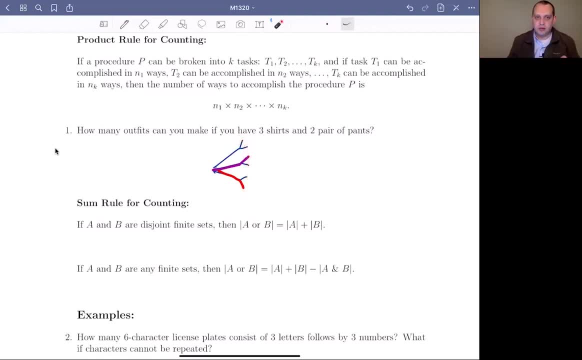 branches. That's kind of the justification that I like to use for the product rule. right, If you have three shirts, two pair of pants, there's six outfits. Three times two is six outfits, So let's just write that down. So three times two. 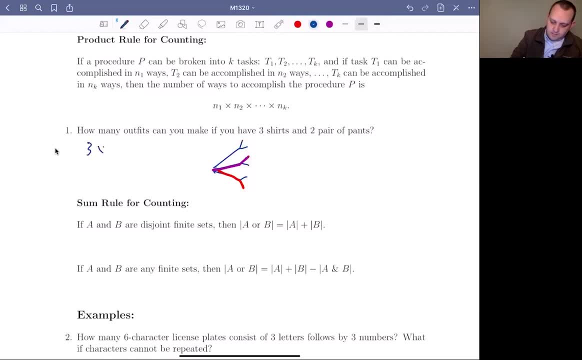 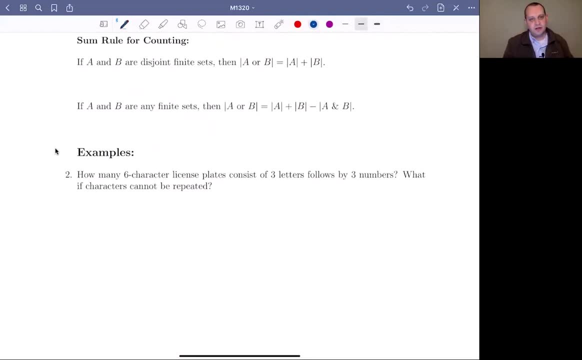 is six outfits. So that's the first rule. That'll already get us pretty far. The next rule is what I like to call the sum rule for counting. Sum meaning addition, the addition rule for counting. It turns out that if you have two sets, 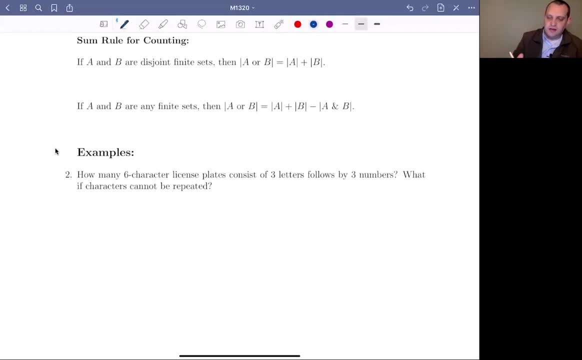 A and B, then the way that you find the number of ways that A or B can happen is you add up the number of ways that A can happen plus the number of ways that B can happen. Let's use blue here, And then you're going to. 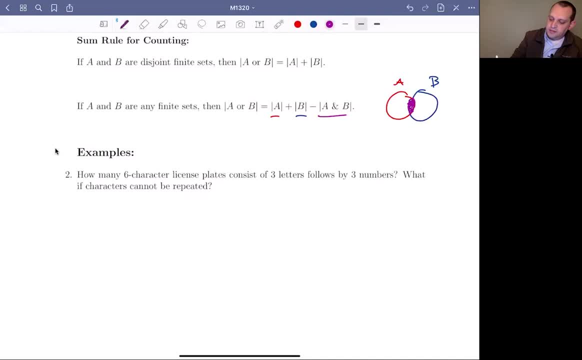 You're going to subtract the number of ways that they both happen at the same time. So you subtract the intersection, And so this is the general rule: If you have an A, If you have an or statement, the way that you handle that, the way that you can count the number of ways that A or B happens. 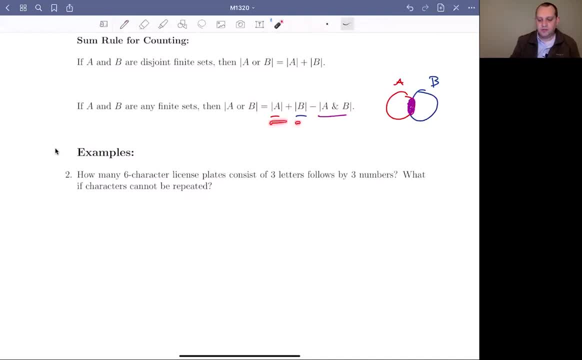 is you count the number of ways that A happens plus the number of ways that B happens, minus the number of ways that A and B happen at the same time. So this is the sum rule for counting As a special case if A and B don't have any elements. 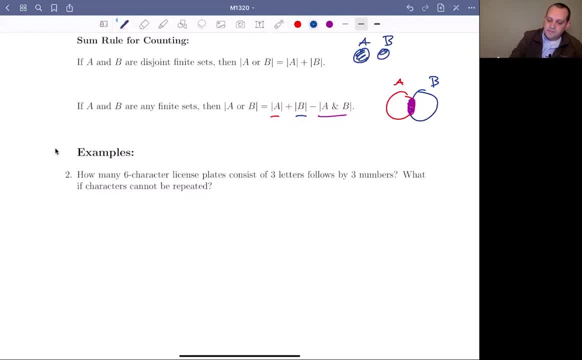 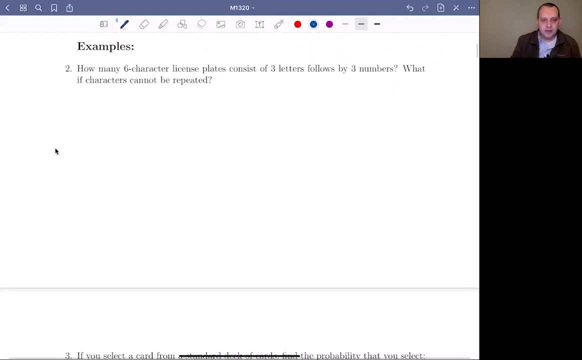 in common so they have no overlap. then you can just add up the number of ways that A happens plus the number of ways that B happens. So that's kind of a special set, a special case of the general rule. So with that in mind, let's go through and let's do some of these examples. 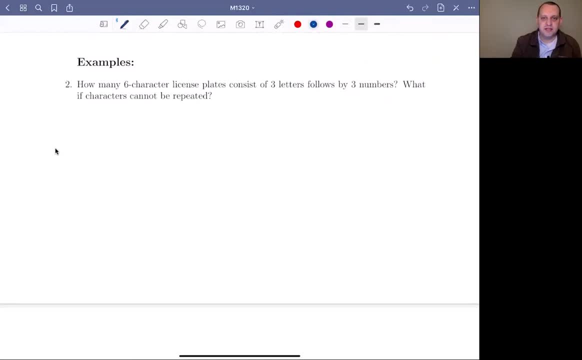 The first example is: I want to think about having a six character license plate. it's going to be three letters followed by three numbers, And I want to know how many ways are there to do that. And so I want to think about how many. 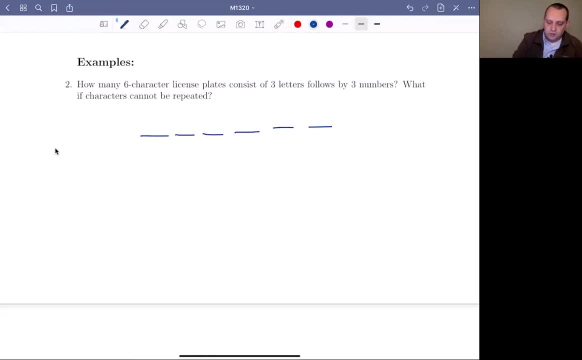 choices do we have for the first letter, second letter and third letter? Well, there's 26 of those, 26 and 26.. So we have 26 choices for the first character, 26 choices for the second, 26 choices for the third, and then we have 10 choices. So 0 through 9, there's 10 digits. 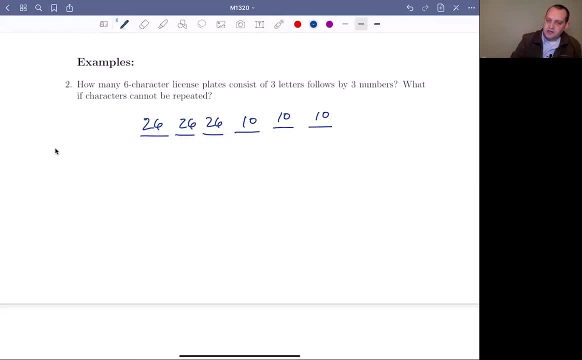 10 choices for the fourth character, 10 choices for the fifth and 10 choices for the sixth character. So altogether there's going to be 26 cubed times 10 cubed, and whatever that is I don't care. So that's how many six character license plates we can have. 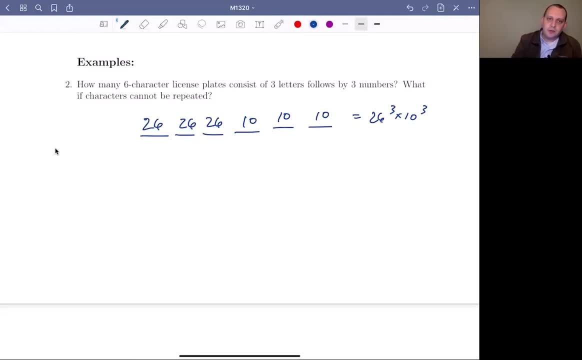 The second part of this is: we want to know what if we're not allowing characters to be repeated. So it's going to be the same sort of calculation: We have 26 choices for the first letter, but if we're not allowing characters to be repeated, then we don't have 26 choices for. 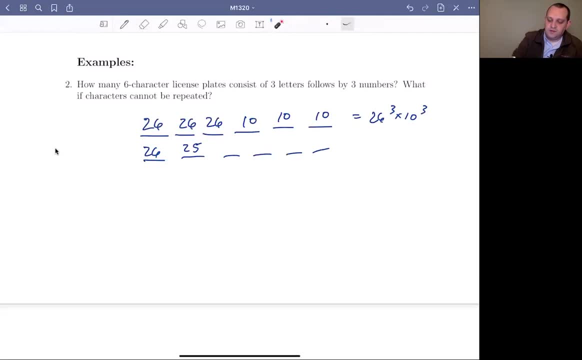 the second letter, We only have 25.. Because whatever that first character is, we can't use it anymore. And likewise, whatever the first two characters are, we can't use those for the third character. So we only have 24 choices for the third character, And likewise we have 10 choices for the first. 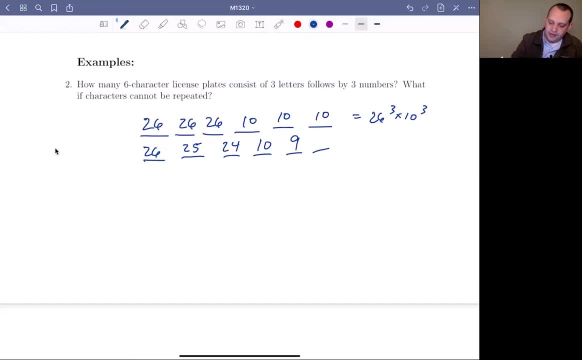 digit, nine for the second digit, eight for the third digit and again, whatever that is, I don't have a nice way to write this, or at least not yet. Times 10 times 9 times 8.. So that's the number of six character-like. 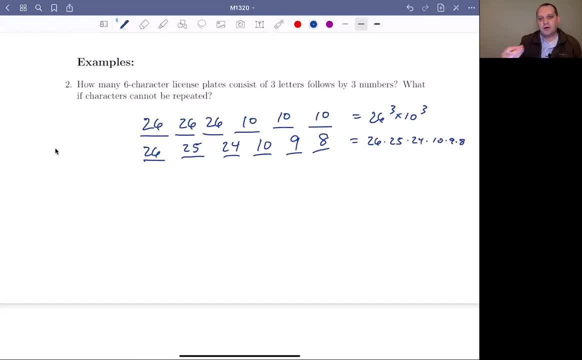 license plates where we have three letters followed by three numbers and we're adding the restriction that no character can be repeated. That's the product rule in a nutshell. I don't really have too much more to say about that. The next example I want to do is from a standard. 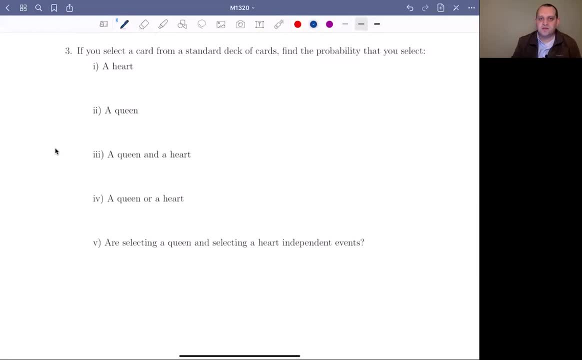 deck of cards. So, just as a reminder, standard deck of cards is 52 cards split into four suits. So the four suits are: clubs, diamonds, hearts and spades. Clubs and spades are black, Diamonds and hearts are red, And then each suit. so those are the four suits, and then each suit has 13. 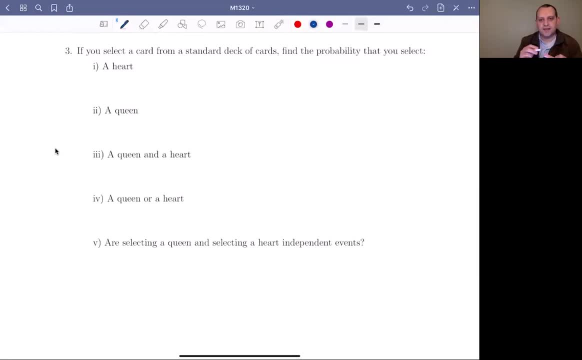 denominations. So there's a, two, three, four, five, six, seven, eight, nine, ten, plus a jack, queen king and ace. Okay so, four suits, 13 denominations. in each suit, 52 cards. 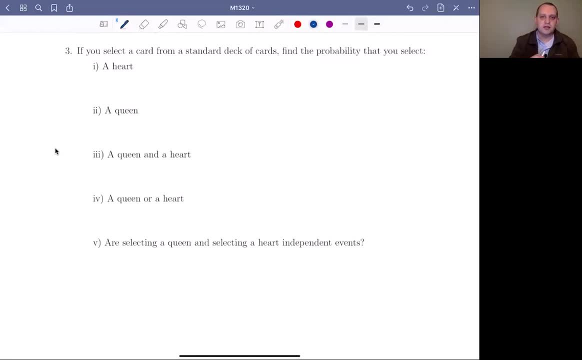 So that's a standard 52 card deck. So what we want to know is: this is a probability question and again it's going to be completely analogous to just counting, but we're going to select one card from the standard deck and we want to know what's the probability that it's a heart. 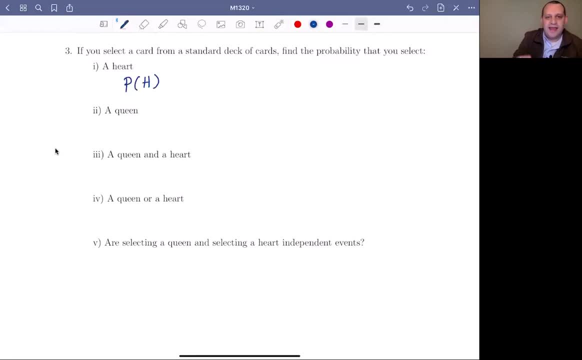 So we want to know what's the probability that it's a heart. I'm going to let h be the event that it's a heart, And so this is going to be the number of cards that we're going to be able to divide by the number of hearts. I'm just going to write this out the first time, Divided by the. 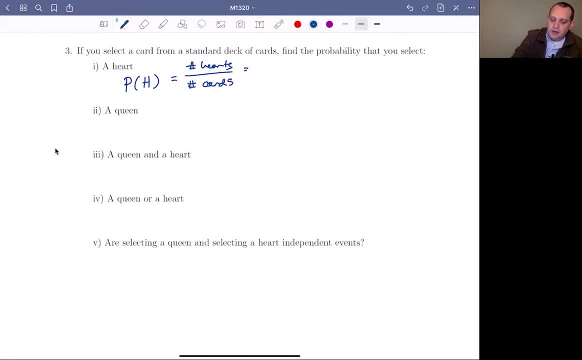 number of card choices that we have, And there's 13 hearts and 52 total cards. So this means that a randomly selected card will be a heart, with probability one-fourth. Okay, what's the probability that we select a queen? Well, how many queens do we have? 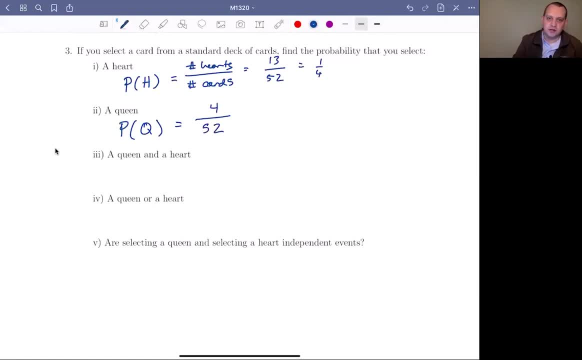 Turns out four. There's one of each suit. Divided by the number of hearts, we have 52 cards, So this is one out of 13.. What's the probability that we select a queen and a heart? How many cards are queens and hearts? One Queen of hearts out of 52.. A queen or a heart? 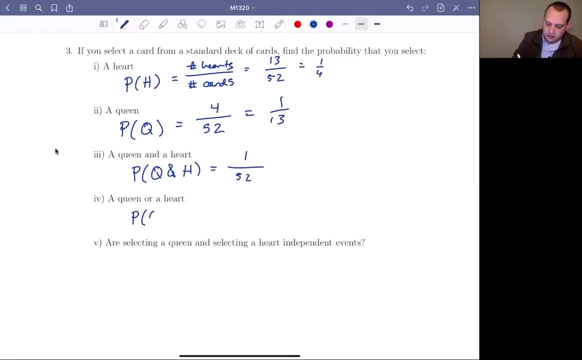 So what we're going to do here is we're going to calculate the probability that we select a queen or a heart, And so that's going to be the probability that we select a queen or a heart. So that's going to be the probability that we select a queen plus the probability that we select a heart. 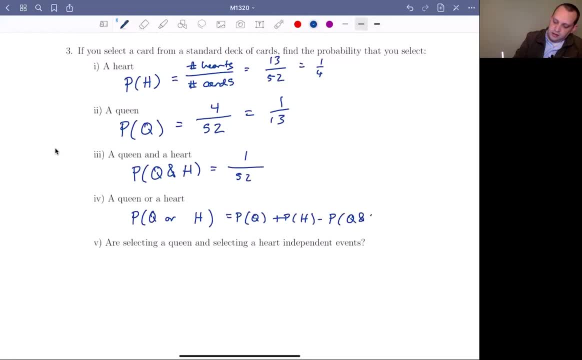 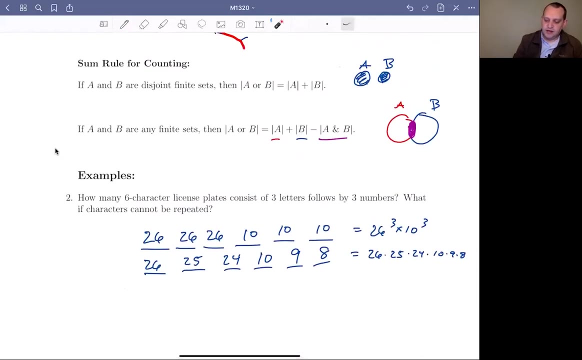 minus the probability that we select a queen and a heart. Notice that the rule that we had up above was actually for counting, but the same rule works for probability for the same reason, Just because if we take each of the, so if we take this previous example and divide each of these by 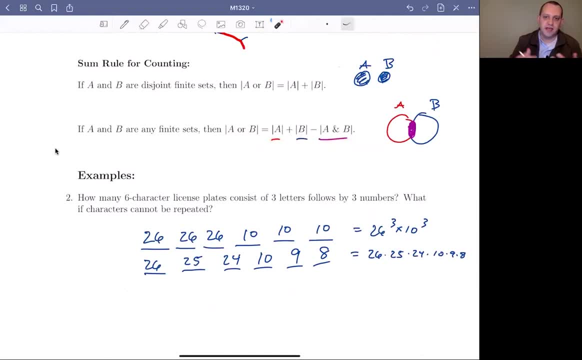 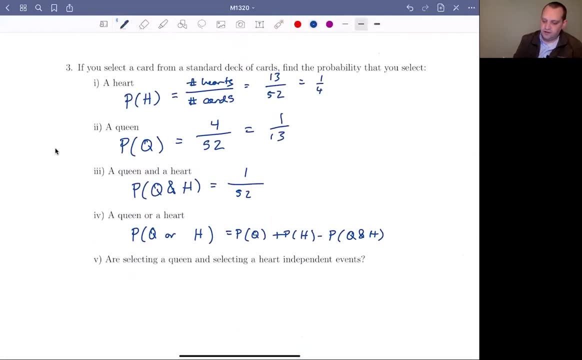 the total size of the sample space. you turn counting sets into probabilities, So really the same rule is going to work for probabilities, So we already have found these. The probability that we select a queen is four out of 52.. The probability that we select a heart is 13 out of 52.. 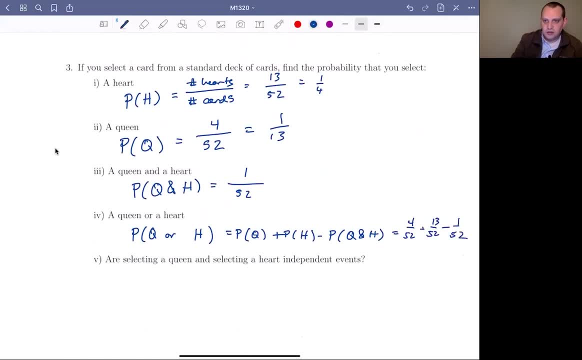 We're subtracting, we're over counting the queen of hearts, And so that's going to be 17 minus one is 16 over 52. And that's four over 13.. If you're into simplifying, I don't care. So probability: 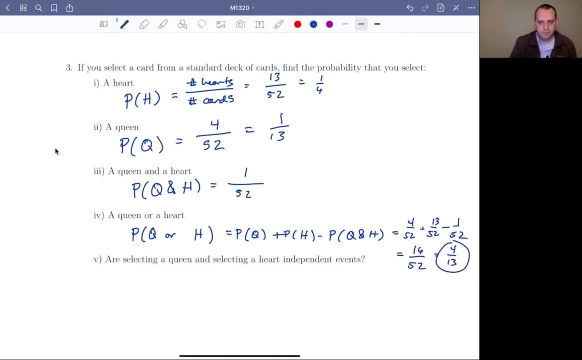 four over 13 is 13 out of 52. And that's four over 13. if you're into simplifying, I don't care So. probability: four over 13 is 13 out of 52. And that's four over 13. if you're into simplifying, I don't care So Ru. 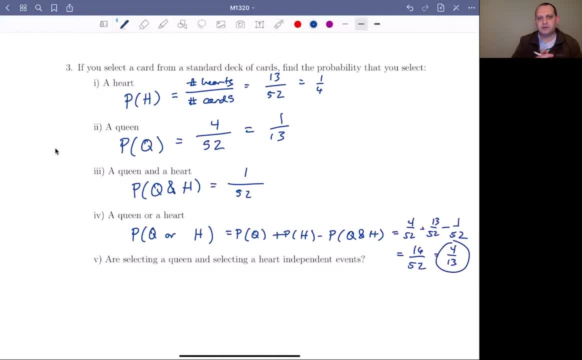 don't you have any use for converting selected events. You don't have to do that. You want to have two or three critical thoughts. If you look at, consider midterms and analysis of Woof shows you the result that comes from our Honestly. 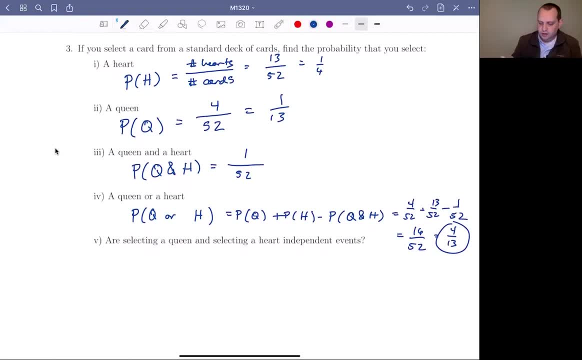 So for those who aren't listening in and are struggling to communicate your inputs, So for those who aren't listening in and are struggling to communicate your inputs, e will help you find that it's also worth considering that you know opening it and 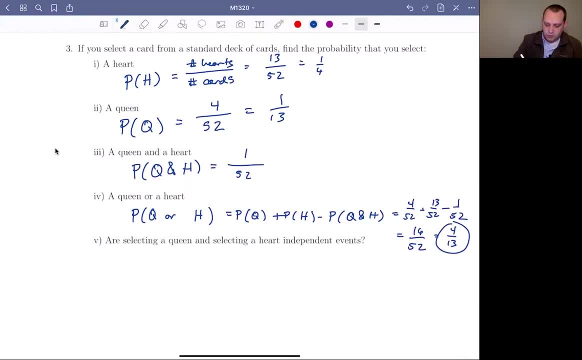 we had a formula for that. so what we want to do is we want to compute, we want to know: are the probability of q and the probability of q given h or yeah, so the probability of q given h? are they equal? okay, so are these two sets equal? let me write this a little better. 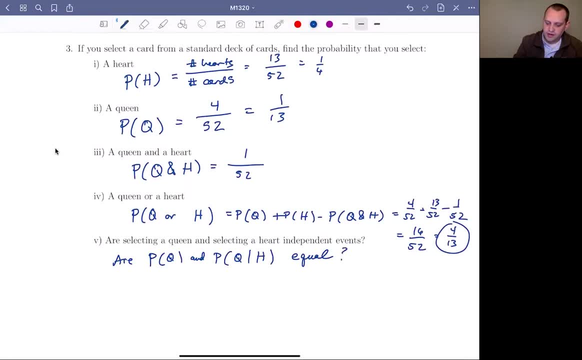 so are those two probabilities equal, and so we have to compute each of these probabilities. now, of course, we computed the probability of selecting a queen. we already know that the probability of selecting a queen was 1 out of 13. okay, that we did in part two. 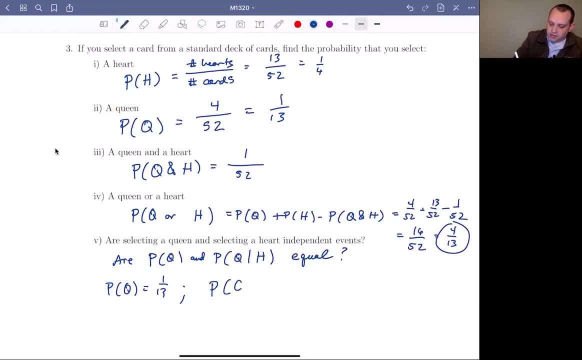 and so now we just have to compute what's the probability that we select a queen, given that we know we've selected a heart, and so, for conditional probabilities, we have our formula that this is the probability of q and h divided by the probability of h, and that's going to be. let's see, q and h, we computed to be 1 over 52.. 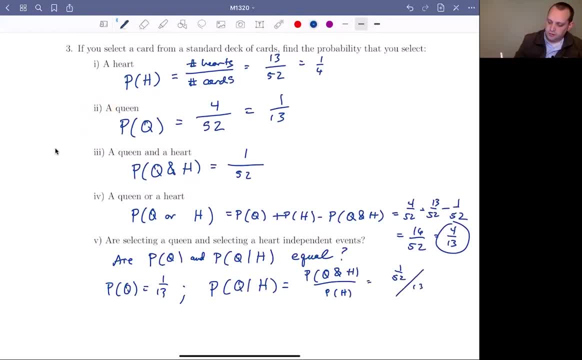 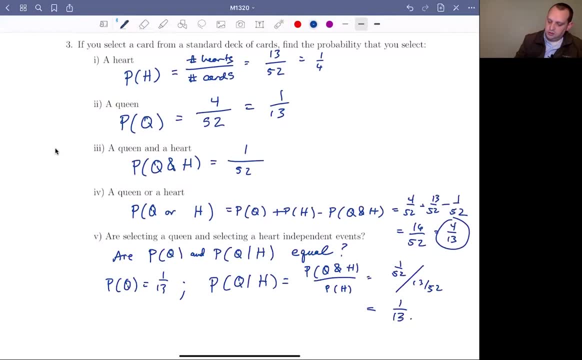 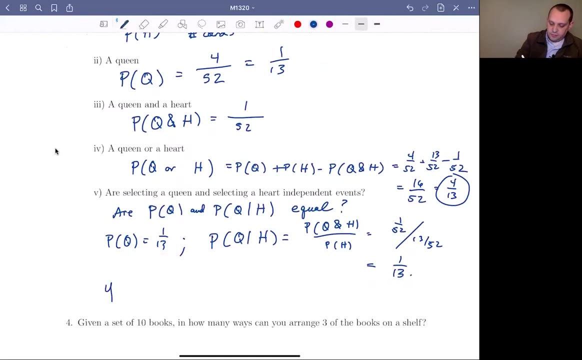 the probability of h is 13 over 52, and so if we divide those, it turns out we get 1 over 13.. so are those two probabilities equal? yes, yes, they are, and so it turns out. are they independent events? yes, okay. q and h. let me write this, just this is clear what we're saying here: q and h are independent. 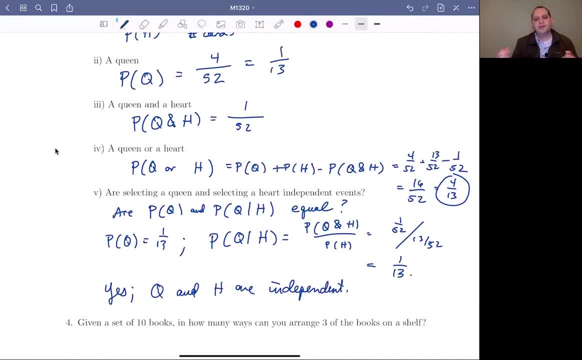 okay, and the way i want you to think about this is that if you were to randomly select a card and you want to know what's the probability that it's a queen, well, that's 4 out of 52. okay, so that's a 1 out of 13.. 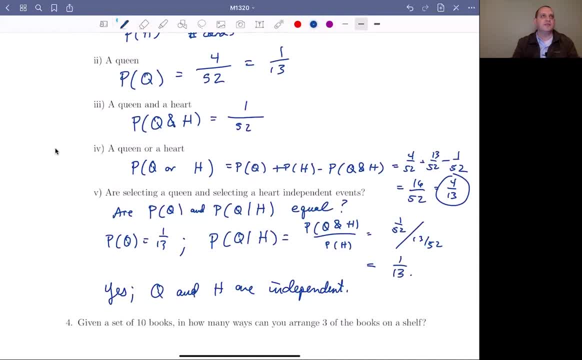 on the other hand, if you know ahead of time that the card that you've selected is a heart, so there's no way you've selected a club or a diamond or a spade. you know it's a heart and then you want to know, given that it's a heart, what's the probability that we've selected a queen? 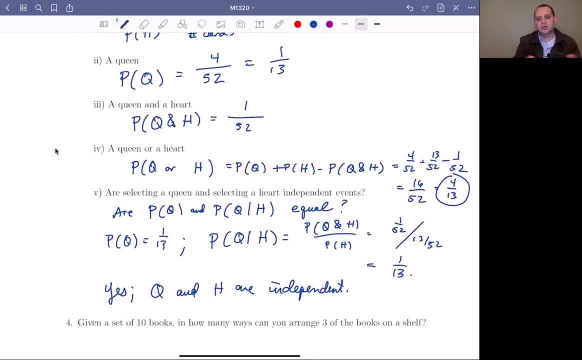 it's still 1 out of 13 or 4 out of 52.. so, knowing that extra bit of information doesn't change the prior probability, okay, so these are independent events. in the next video we'll talk about arranging and choosing sets.